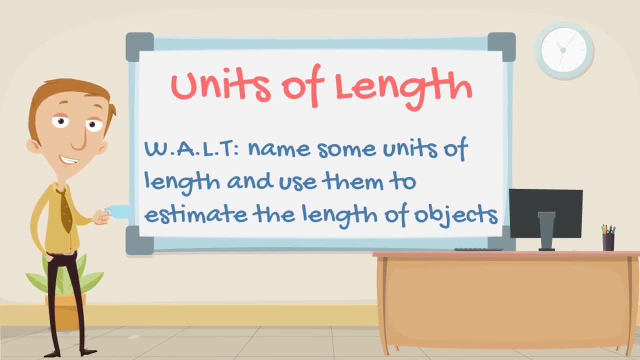 Hello and welcome back to Wrongmar. In today's maths lesson we're taking a first look at the units of length. Our wall for today is to name some units of length and to use them to estimate the length of different objects. But first, what does that word length mean? When I ask you about 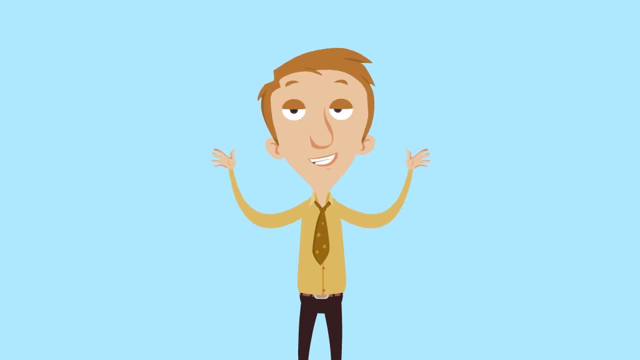 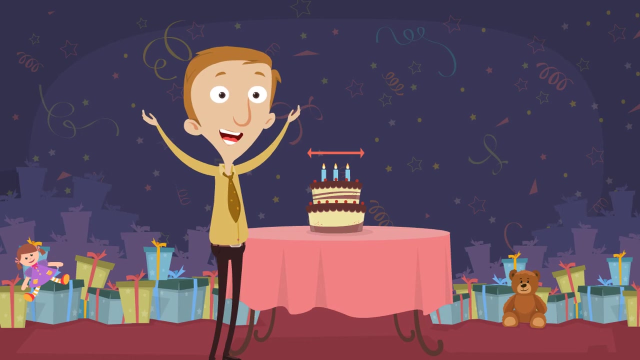 length. what am I even talking about? Pause the video and see if you can write down what length means. Well, when we talk about length, we're talking about the distance from one place to another or from one point to another. That could mean the distance from one side of a cake to the. 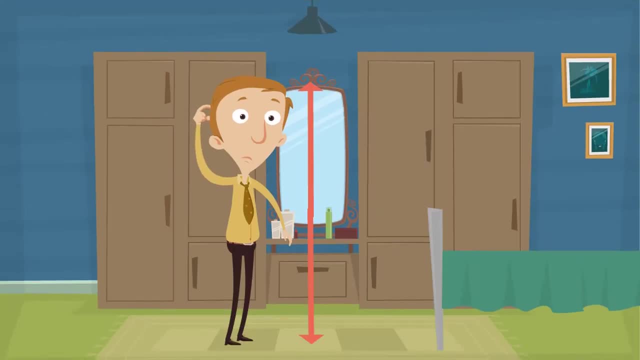 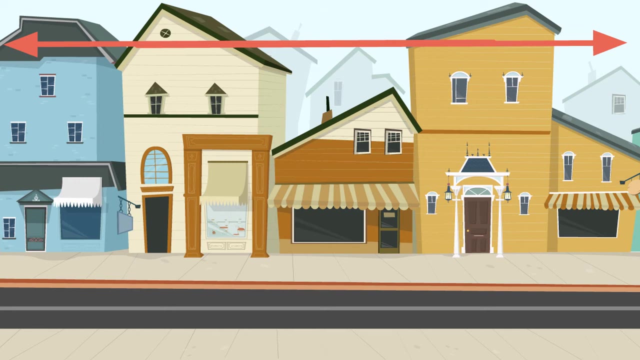 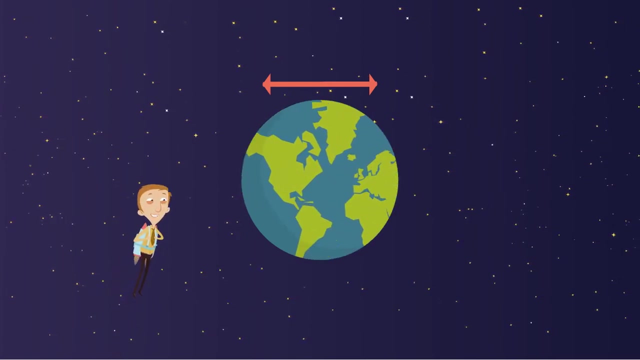 other side of the cake. It could mean the distance from my toes up to my head. We could be talking about how far I can run. That could be a length. Or we could be talking about something huge like the distance from one side of the earth. 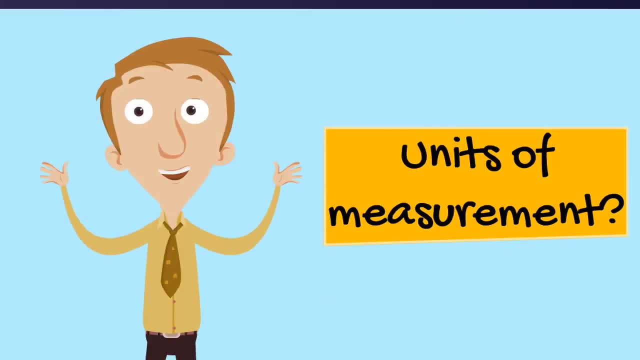 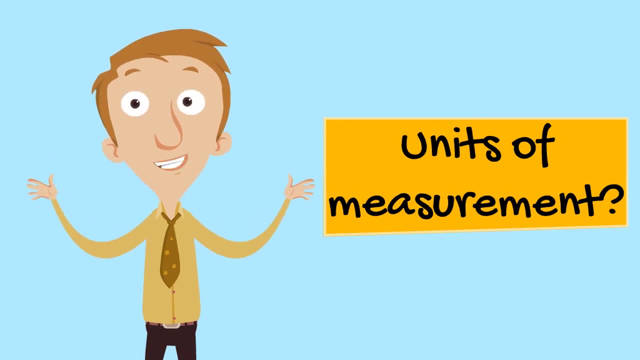 to the other side of the earth. Depending on what we're measuring, we'll need to use a different unit of measurement for length. Do you already know any of the units of measurement for length? Pause the video and write down an answer. Did you think of these? We have. 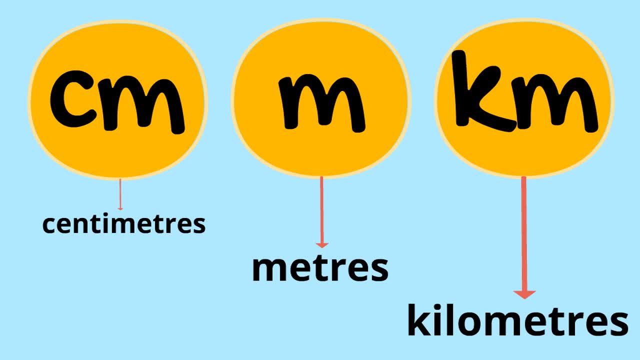 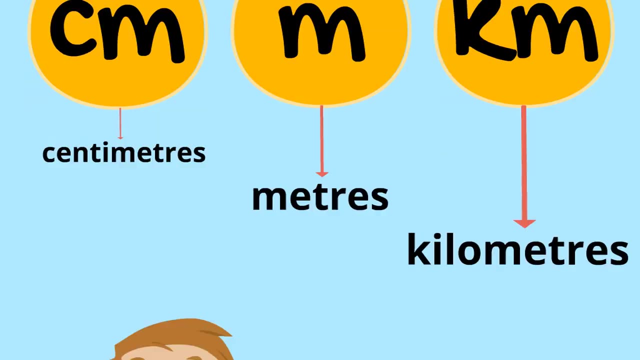 CM, which stands for centimeters, We have M, which stands for meters, And we have KM, which stands for kilometers. We use different units of measurement to measure different things. Let's start off with centimeters. Would you be able to think of something that? 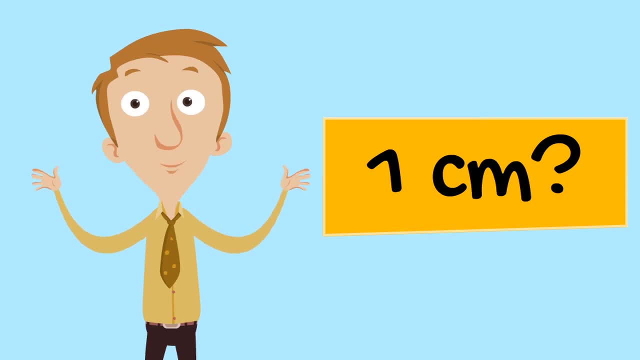 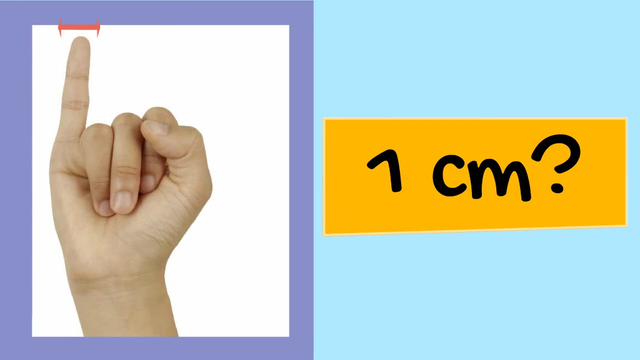 is one centimeter long. Pause the video and see if you can think of something that is only one centimeter. Well, a good way to remember how long a centimeter is is by holding up your hand, looking at your little finger or your pinky finger and seeing how far it is. 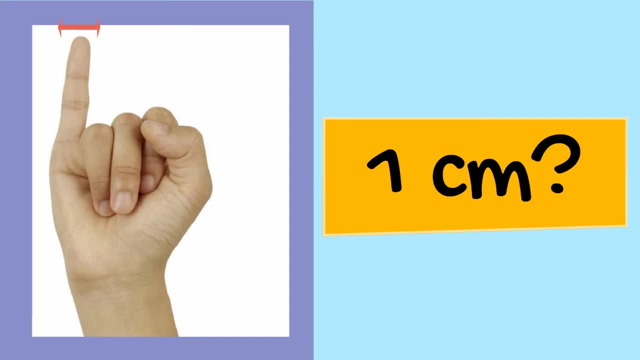 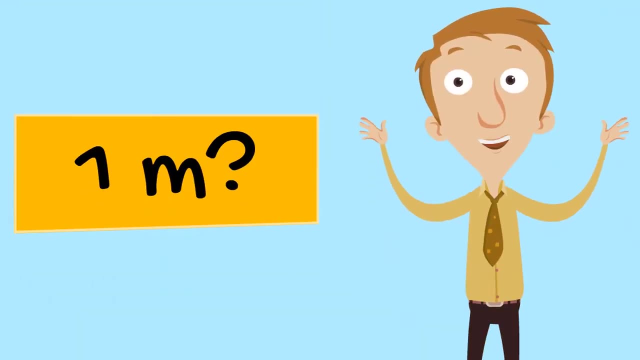 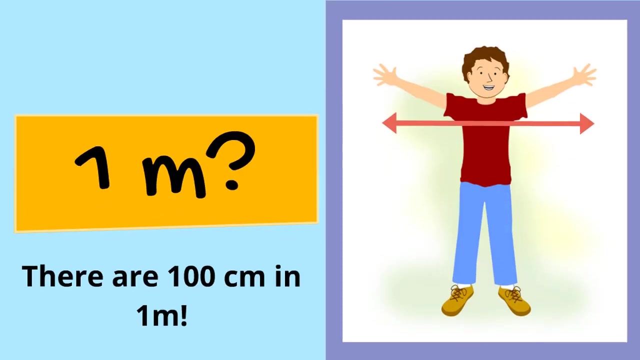 from one side of your pinky to the other side of your pinky. That's roughly about one centimeter. Okay, How about a meter? Can you think of any way of showing how big a meter would be? Pause the video and write down an answer. Well, a meter is quite a bit bigger than a centimeter. 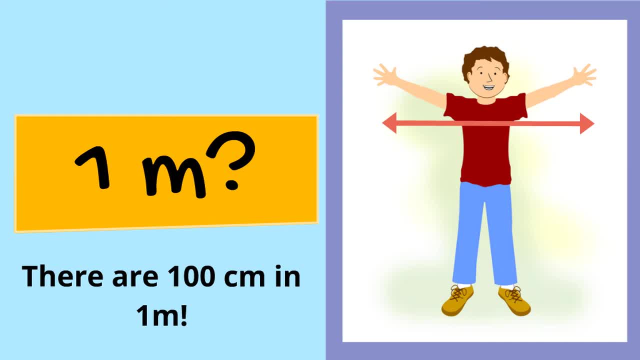 In fact, there are hundred centimeters in one meter, So that means there's a hundred pinky fingers beside each other. to make this measurement, The best way to think of one meter is to stretch your arms out to the side and roughly from. 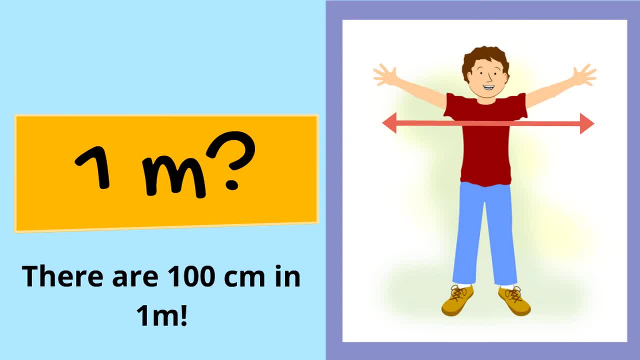 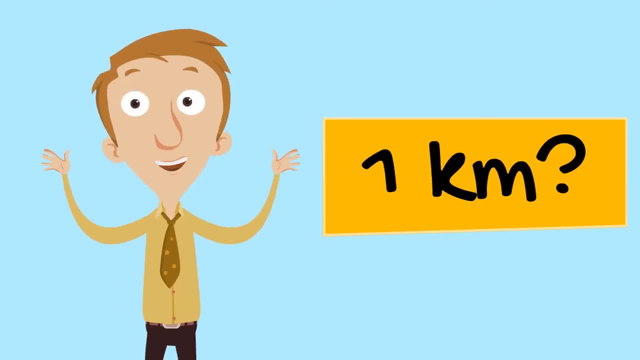 one hand to the other in a straight line across is one meter. How about a kilometer, our biggest unit of measurement today? How far do you think a kilometer would be? Pause the video and write down an answer. Well, let me tell you, one kilometer is big There. 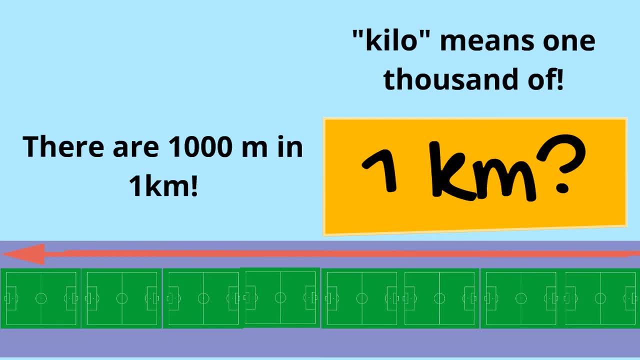 are one thousand meters in a kilometer. That means imagine a thousand children in a kilometer. One thousand children standing beside each other with their arms stretched out. Or if you can picture how big a football pitch is, one kilometer is ten football pitches. 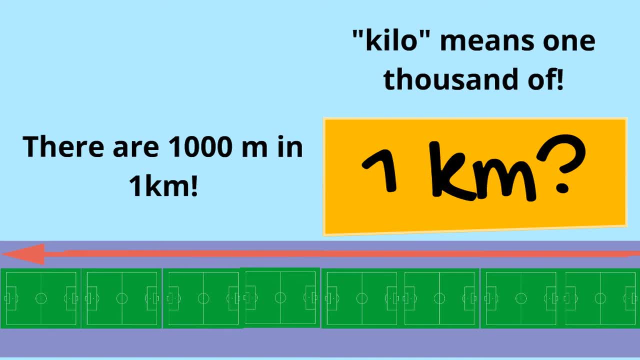 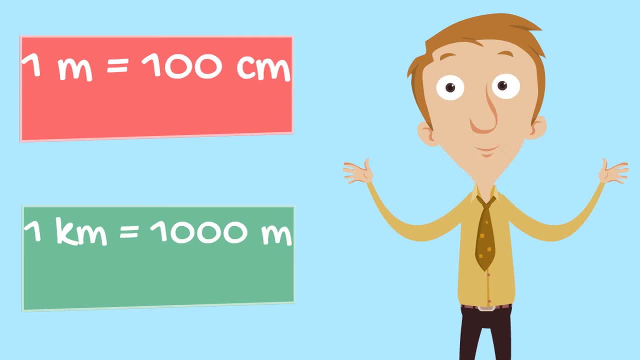 in a big long row. That's so many pitches they don't even fit onto this screen. Okay, so one meter is equal to one hundred centimeters And one kilometer is equal to one thousand. Remember that. That's a very important fact for today. 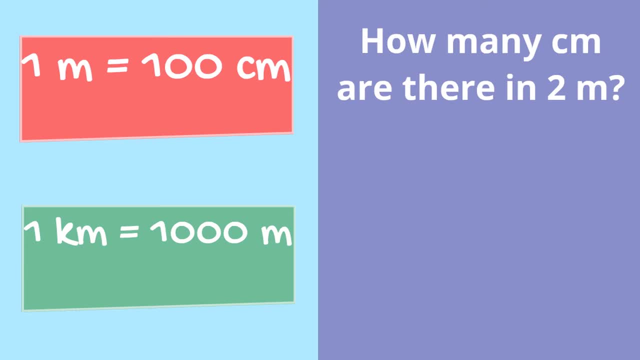 If you know those facts, how many centimeters would there be in two meters? Pause the video and write down an answer. Well, if there's one hundred in one meter, then there must be two hundred in two meters. So the answer is two hundred centimeters. 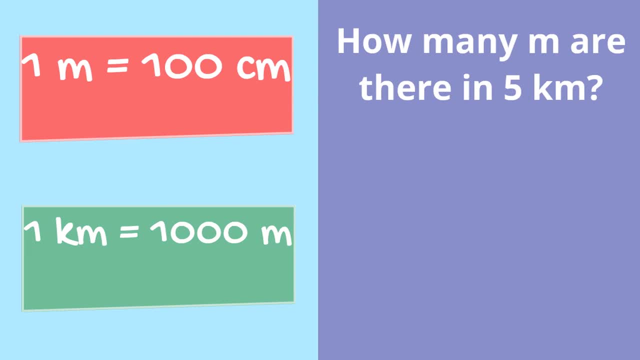 How about this one? How many meters are there in five kilometers? Pause the video and see if you can figure out the answer. Well, if there is one kilometer is equal to one thousand meters, then five kilometers is going to be equal to five thousand meters, Okay. 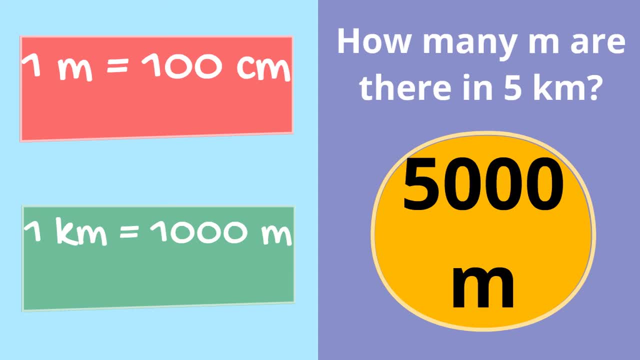 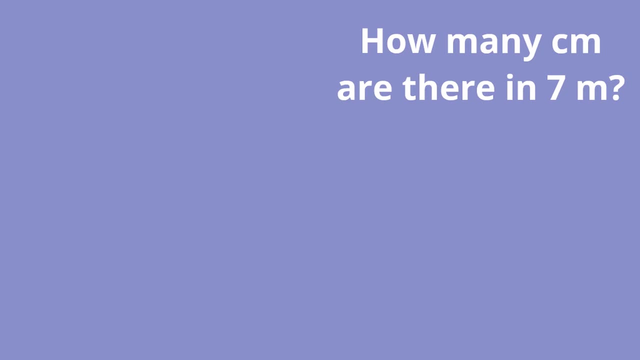 I'm going to make it a little bit harder for you now. I'm going to get rid of the facts here. If you think you're going to need them, maybe write them down on a piece of paper before going into the next ones. Okay, here we go. How many centimeters are there in seven? 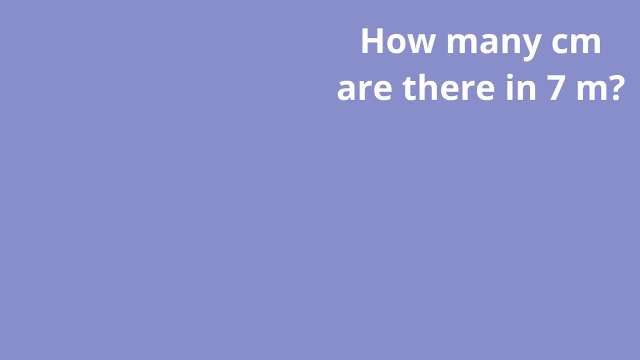 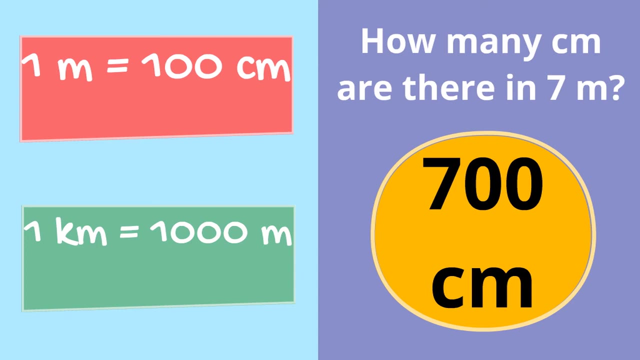 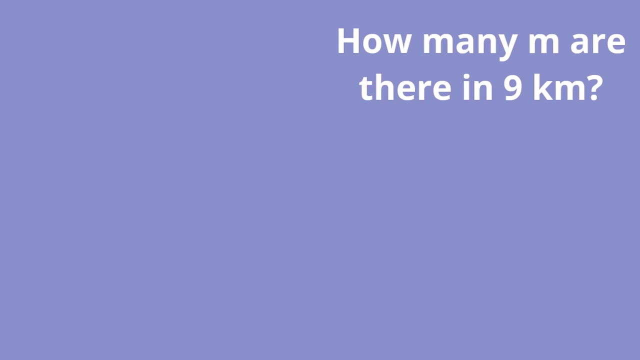 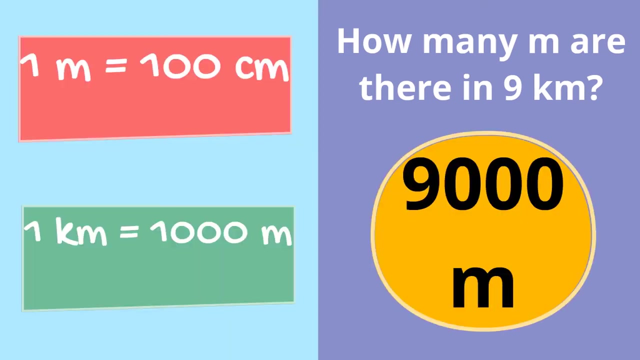 meters. Pause the video and write down an answer. The answer is seven hundred centimeters. Next question: How many meters are there in nine kilometers? Pause the video and write answer. Well, the answer is 9,000 metres. Did you get both of them correct? If you did good job. 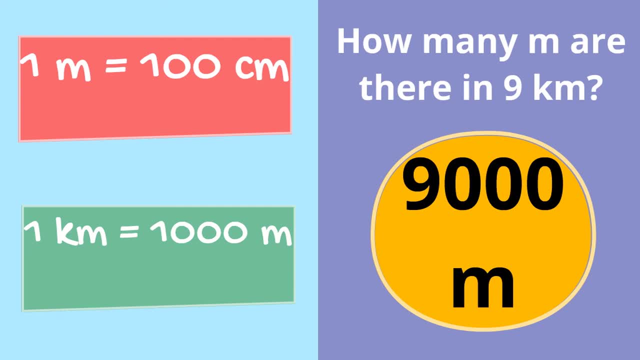 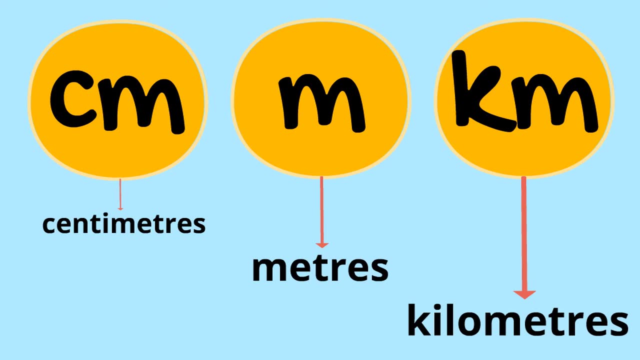 If not, maybe pause the video rewind and have a look at that section again. So, as you probably noticed by now, centimetres are the smallest unit we've talked about today, Meters are the middle unit we talked about today and kilometres are the biggest unit of length. we 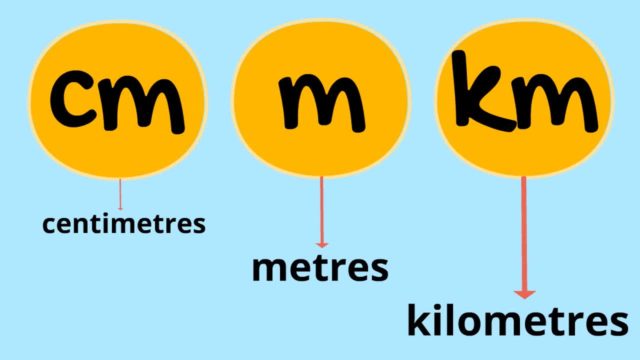 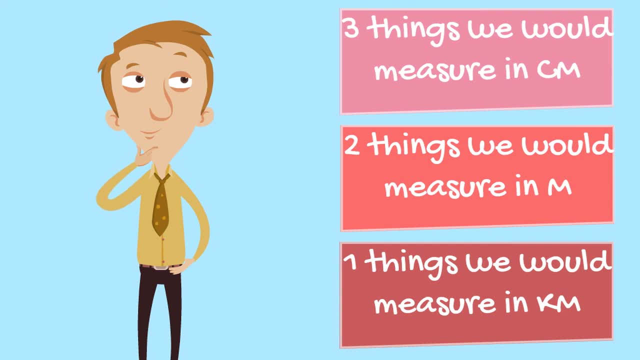 talked about today. Take a look around the room When you're ready. I want you to go grab three things that you measure in centimetres. I want you to touch two things you would measure in metres, and then I want you to stop and think. 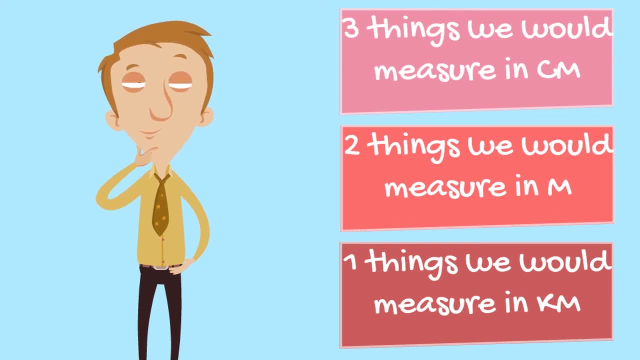 Think of one thing we would measure in kilometres. So grab three things that are measured in centimetres, touch two things measured in metres and pause and think of one thing measured in kilometres. If you want an extra challenge, get a stopwatch out and see if you. 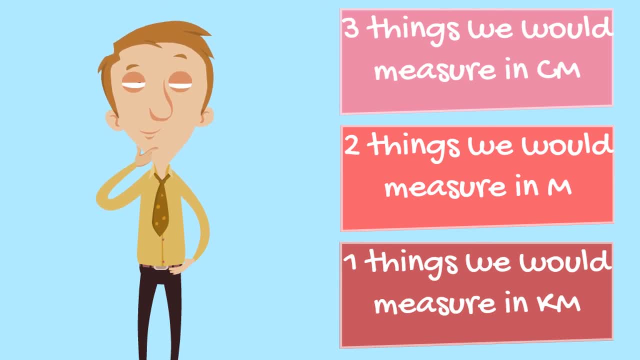 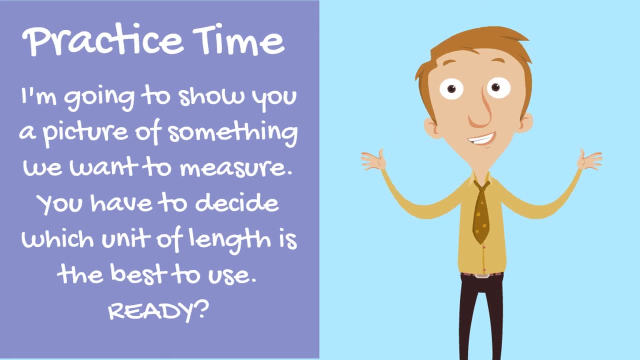 can do it in 30 seconds. When you're ready, pause the video and off you go. Okay, now that you're all experts on centimetres, metres and kilometres, it's practice time. I'm going to show you a picture. 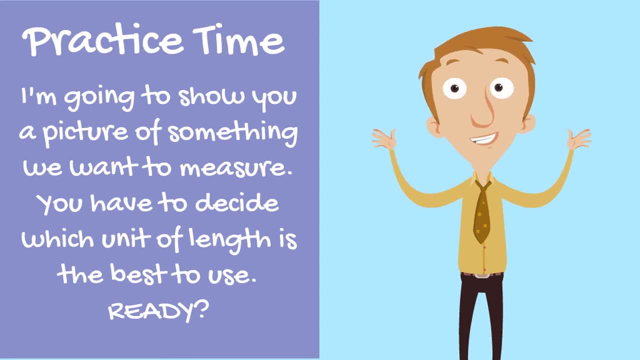 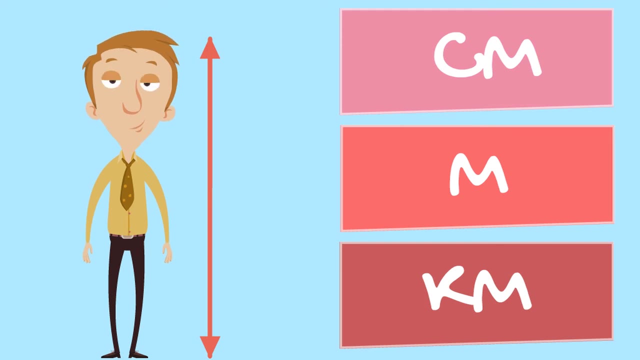 of something that we want to measure. You have to decide which unit of length is the best one to use. Are you ready? Okay, first one: I want to measure my height. If I was trying to measure my height, would I use centimetres, metres or kilometres? Pause the video and write down an answer.